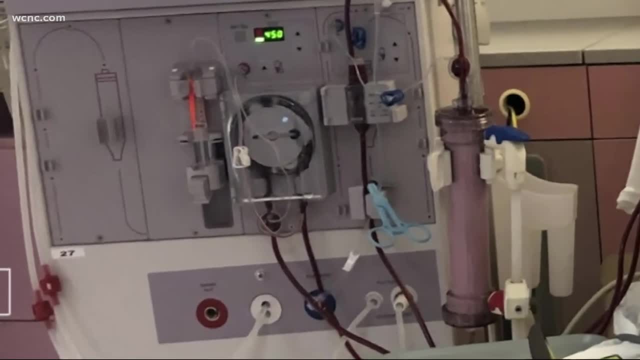 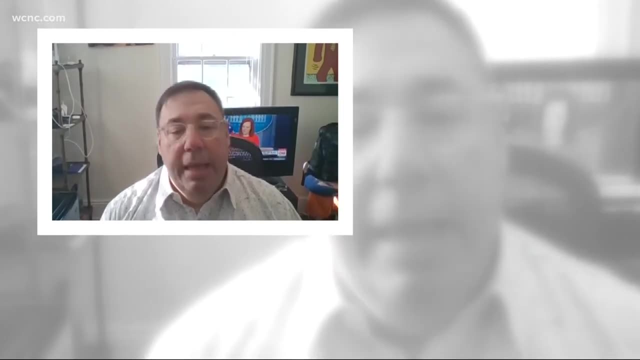 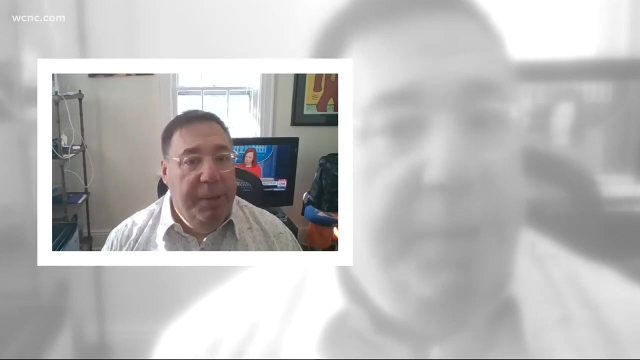 Four hours a day, three times a week, A process that keeps Mark alive. It's afterwards can be very debilitating, And when I mean debilitating, I can be very tired, very cold both, And on occasion, you know, you become worn out. Mark, an old friend who worked with me in news back in Reno, 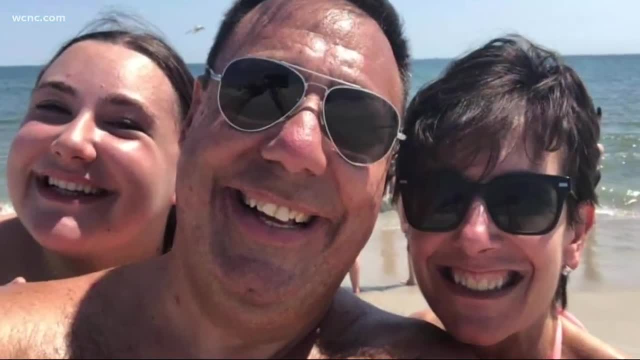 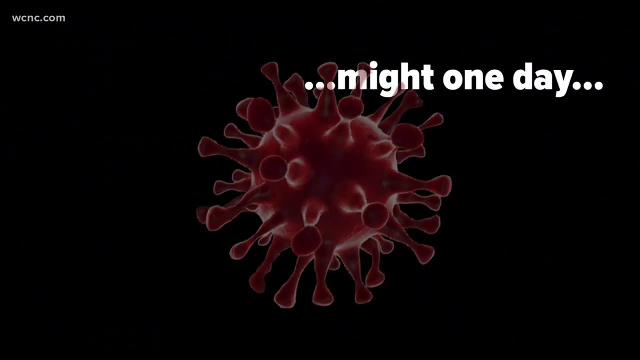 in the early 90s needs a kidney. His story even told front and center in time, square up on that billboard. More on Mark in a moment, But first the process and program that has struggled through COVID, the program that might one day save Mark's life and many others. 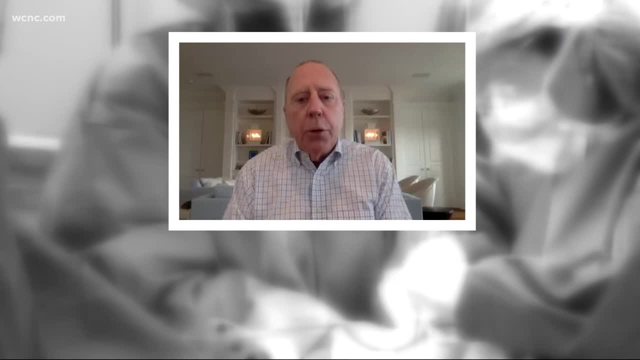 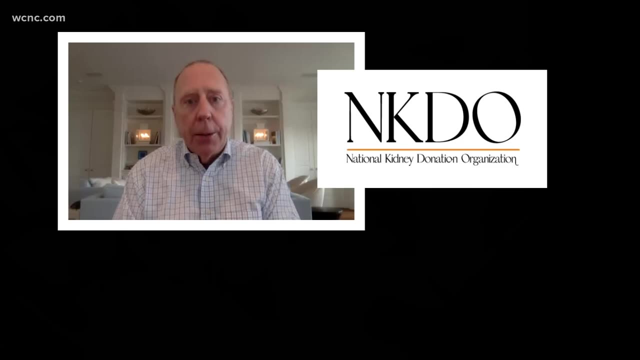 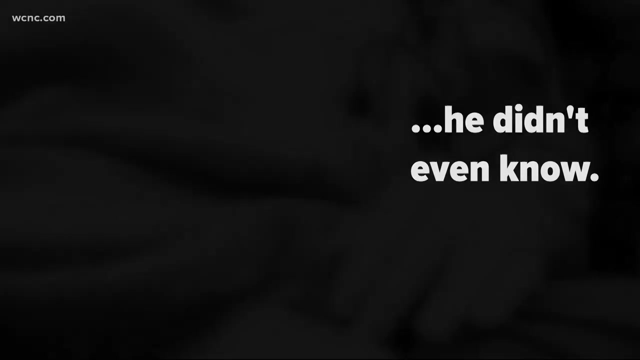 When COVID first hit the transplant center industry across the country shut down. Ned Brooks is the founder of the National Kidney Donation Organization. Ned made the selfless act of donating a kidney. the recipient a young mother. he didn't even know. That process is called a living donor. 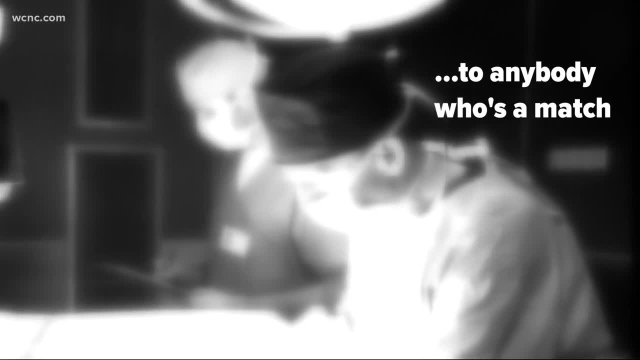 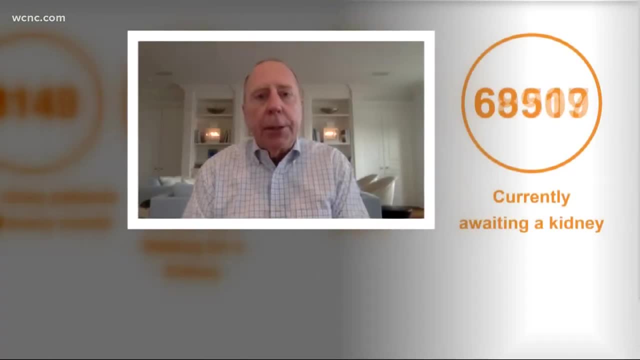 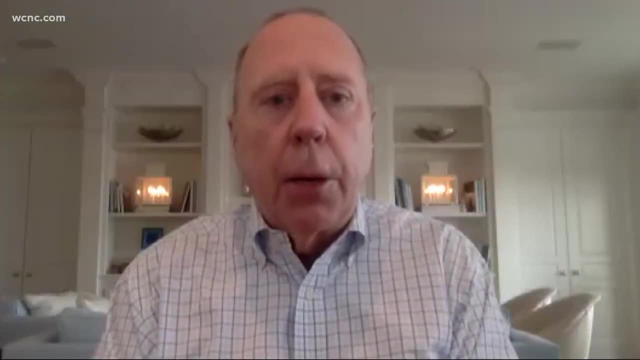 It's a program that allows the donor to be tested and donates a kidney to anybody who's a match, even if it's not the person they want to directly help. You've got about 100,000 people on the waiting list. You've got about 13 people who die from failed kidneys every day. Those numbers we're going to find have gone up dramatically in 2020.. 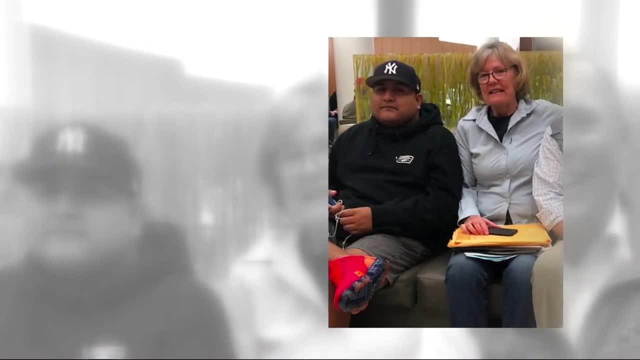 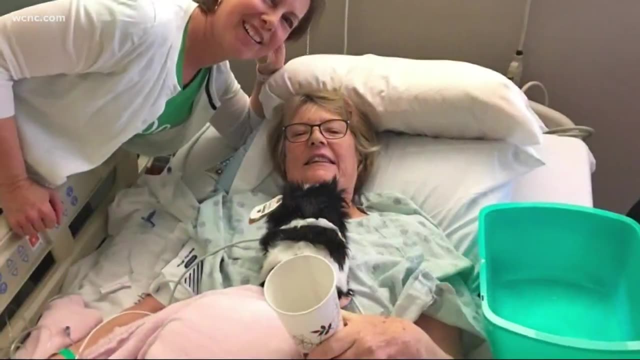 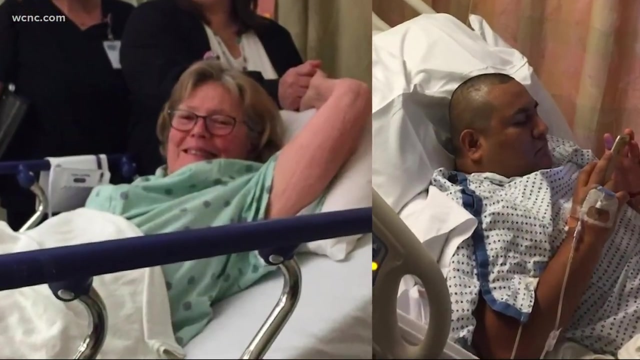 Michelle Hughes in North Carolina told me her son in his mid-20s needed a kidney. When she learned about the living donor program, she jumped in. At 73 years old, Michelle donated a kidney and received a voucher for her son, Dan, who was in end-stage renal disease. A match for him was then found. You might say Michelle saved two lives. 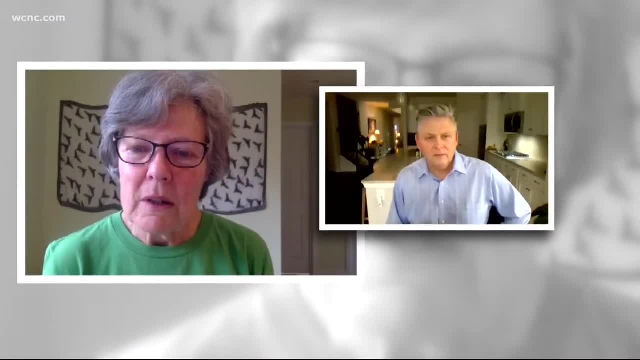 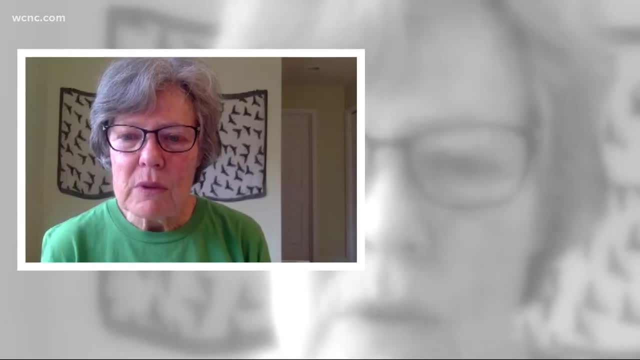 And it's a wonderful gift, And it's a gift for you. It's a gift for you: My life. I just can't tell you what a wonderful feeling it is to have been able to save my son's life Back in New York, Mark Weiner.